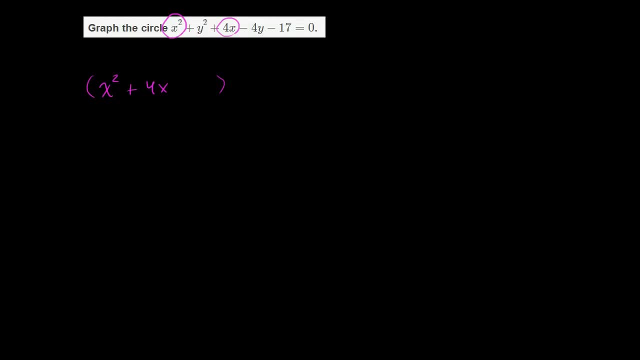 And then I have my y terms. I'll circle those in. Well, the red looks too much like the purple. I'll circle those in blue y squared and negative 4y. So we have plus y squared, minus 4y. 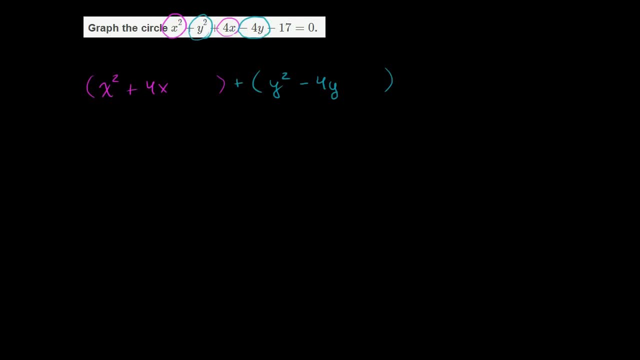 And then we have a minus 17.. And I'll just do that in a neutral color. So minus 17 is equal to 0.. Now what I want to do is make each of these purple expressions perfect squares. So how could I do that here? 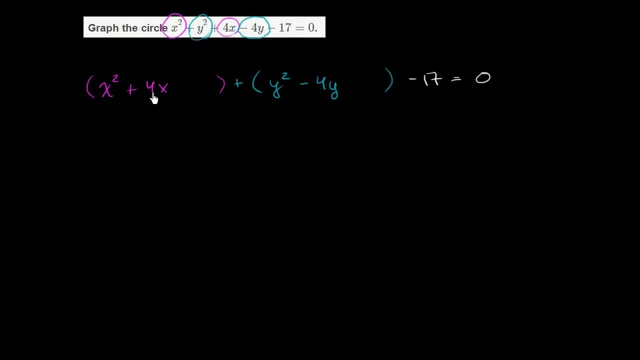 Well, this would be a perfect square if I took half of this 4 and I squared it. So if I made this plus Plus 4, then this entire expression would be x plus 2 squared, And you can verify that if you like. 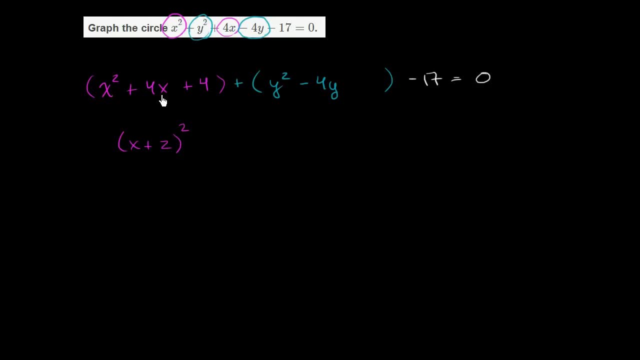 If you need review on completing the square, there's plenty of videos on Khan Academy on that. All we did is we took half of this coefficient and then squared it to get 4.. Half of 4 is 2, squared to get 4.. 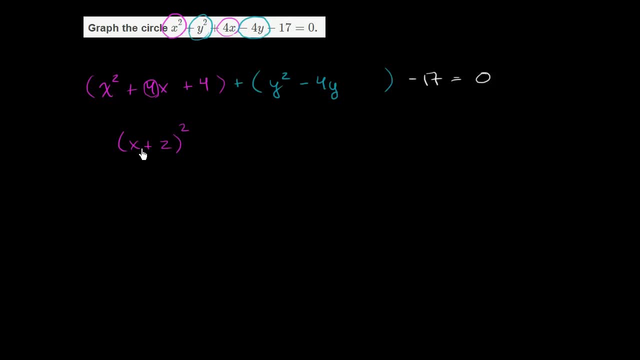 And that comes straight out of the idea. If you take x plus 2 and square it, it's going to be x squared plus twice the product of 2, and x plus 2x Plus 2 squared. Now we can't just willy-nilly add a 4 here. 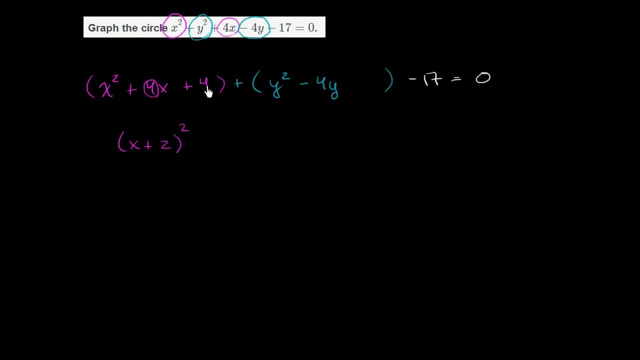 We had an equality before And just adding a 4, it wouldn't be equal anymore. So if we want to maintain the equality, we have to add 4 on the right-hand side as well. Now let's do the same thing for the y's. 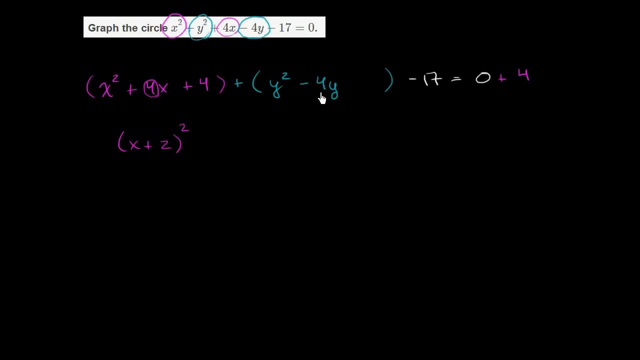 Half of this coefficient right over here is a negative 2.. If we square a negative 2, it becomes a positive 4.. We can't just do that on the left-hand side, We have to do that on the right-hand side as well. 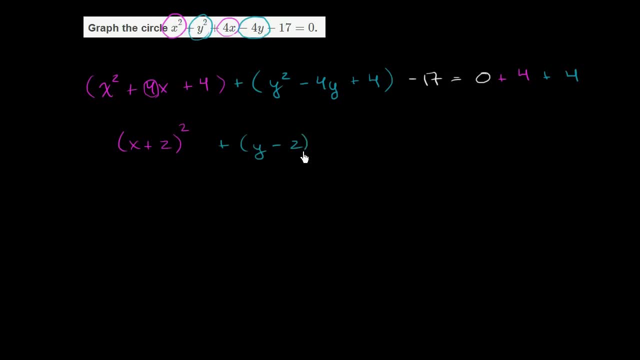 Now what we have in blue becomes y squared, y minus 2 squared, And of course we have the minus 17.. But why don't we add 17 to both sides as well, to get rid of this minus 17 here? 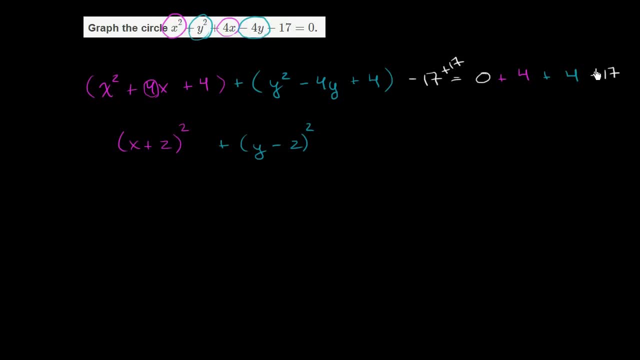 So let's add 17 on the left and add 17 on the right. So on the left we're just left with these two expressions, And on the right we have 4 plus 4 plus 17.. Well, that's 8 plus 17,, which is equal to 25..